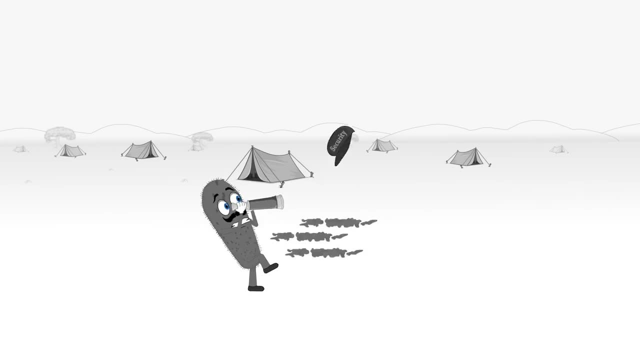 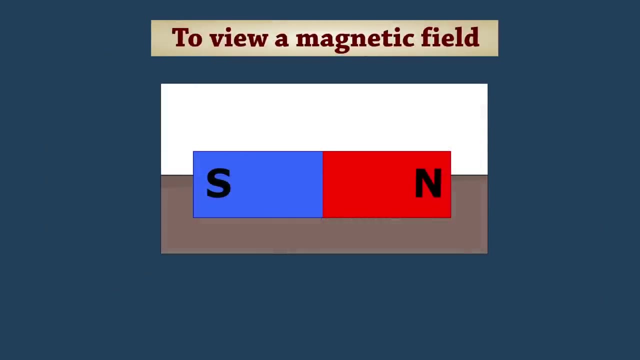 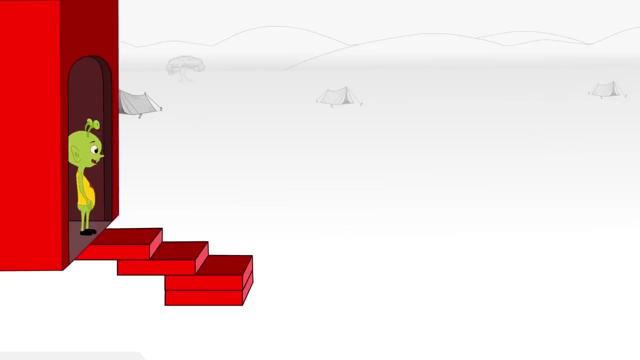 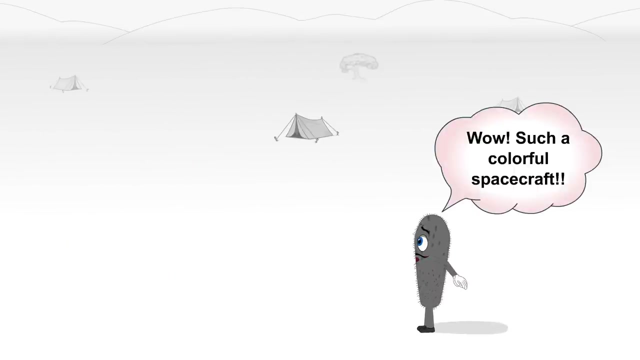 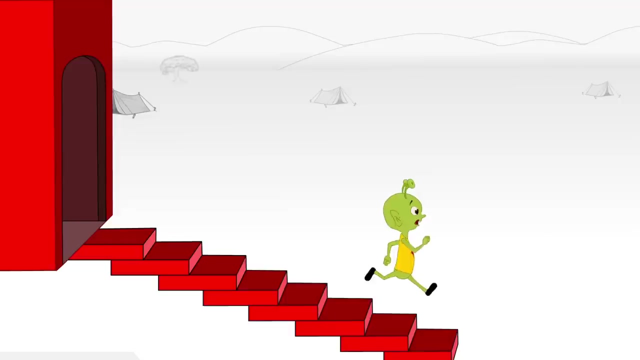 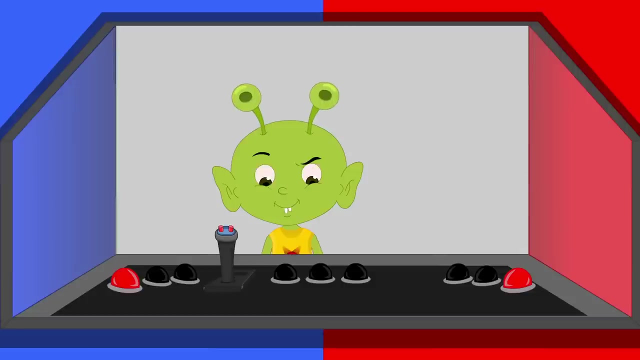 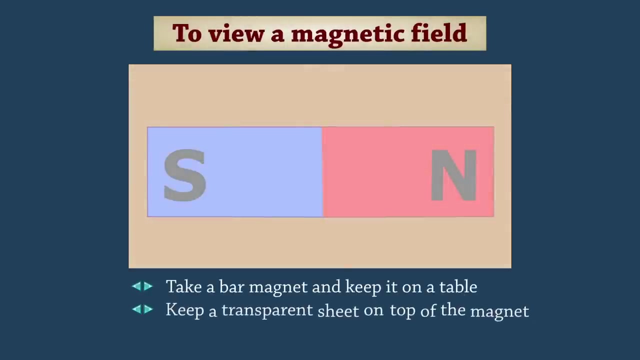 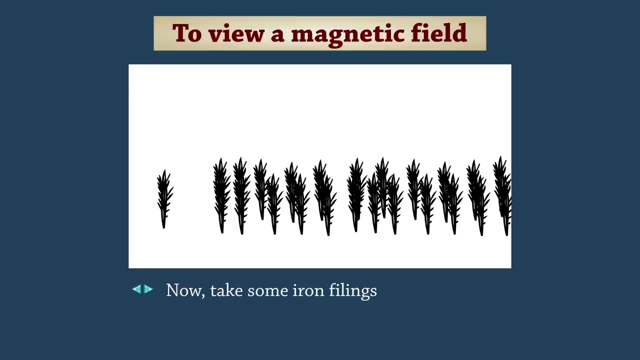 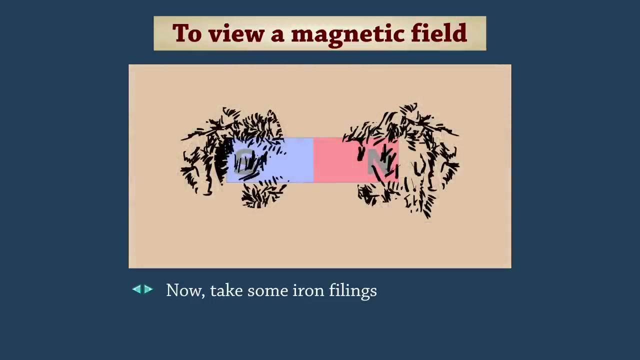 Run. Take a bar magnet And keep it on a table. Wow, Such a colorful spacecraft. Let's go there. Activating transparent sheet. Keep a transparent sheet on top of the magnet. Now take some iron filings And sprinkle them on the paper. 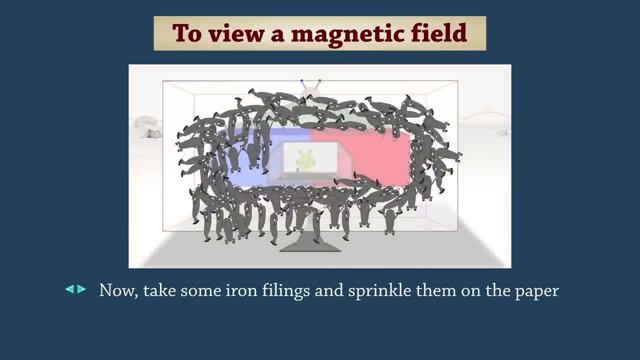 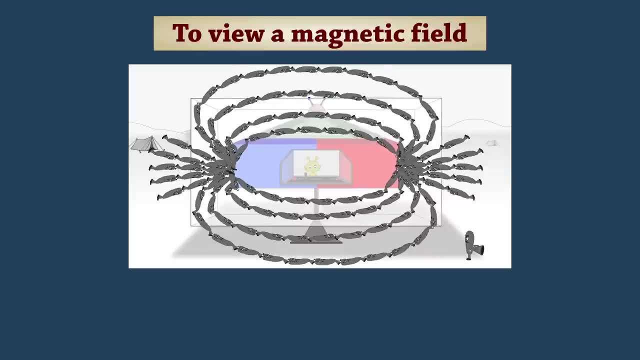 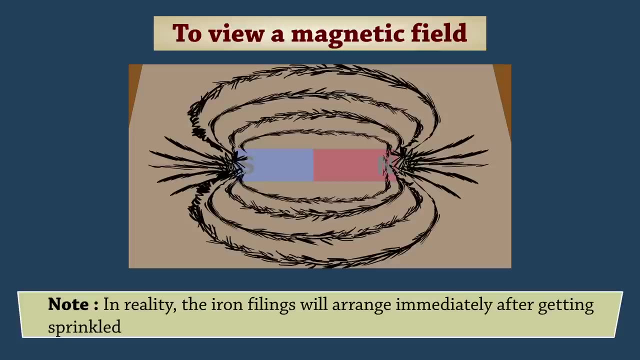 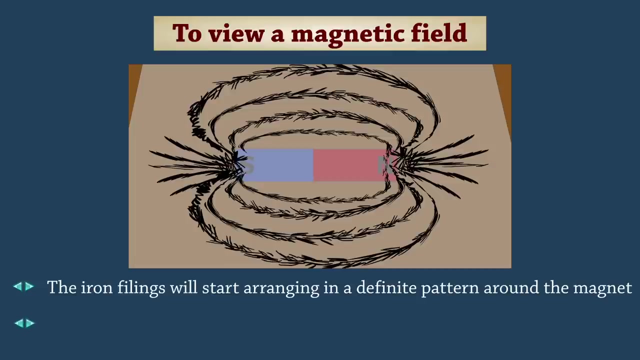 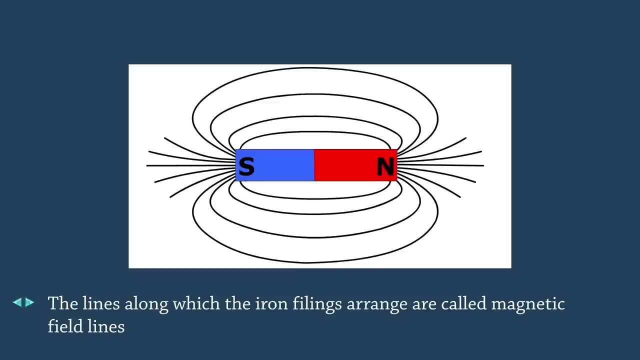 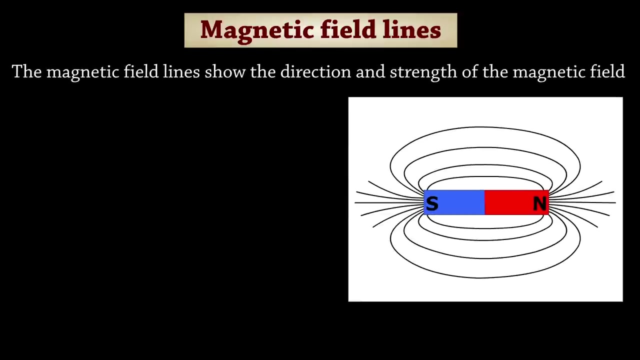 Arrange yourselves properly, The iron filings will start arranging in a definite pattern around the magnet. This pattern is called a magnetic field. The lines along which the iron filings arrange are called magnetic field lines. The magnetic field lines show the direction and strength of the magnetic field. 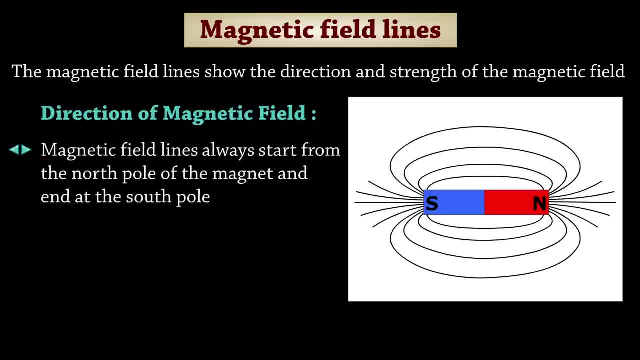 Magnetic field lines always start from the north pole of the magnet and end at the south pole. Soviet law explains magnetic field but will continue to increase the distance to the north pole Inside the magnet. their direction is from the south pole to the north pole.